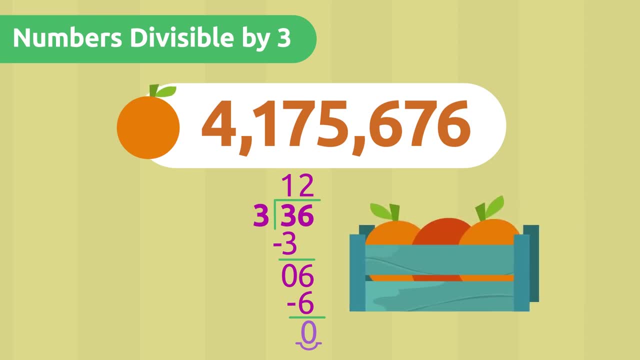 That means thirty-six is divisible by three, Since thirty-six is the result of adding the oranges. applying the divisibility rule of three means that there will be none left over if we pack three in each box. But what happens if we add the digits of a number and we get a very huge number? 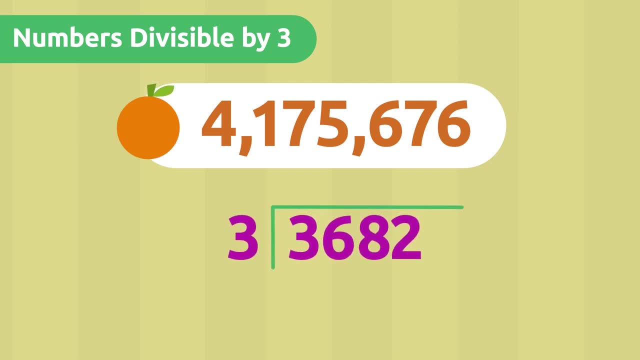 Doing division with such a large number would take us a long time, and what we want to know quickly is the divisibility of a number. In that case, after adding up the digits of the original number, we would go back and add again the digits of that number. 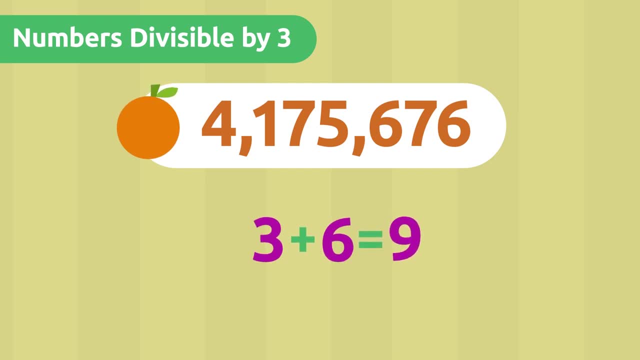 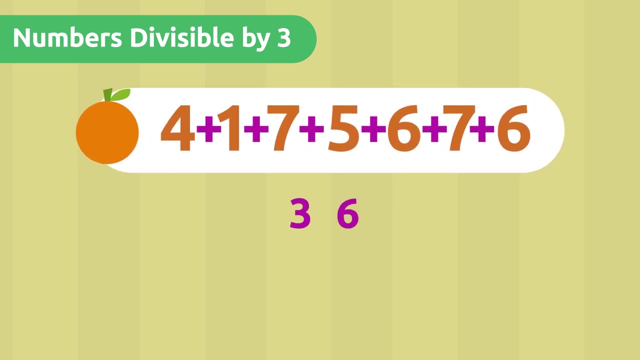 which we have obtained as a result to get a smaller number. If we get a number divisible by three, then the original number should also be divisible by three. When we added the number of oranges, we got thirty-six. If we add up the digits of thirty-six, we should have a number divisible by three. 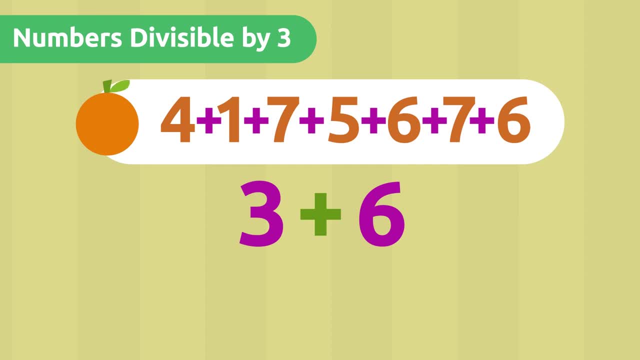 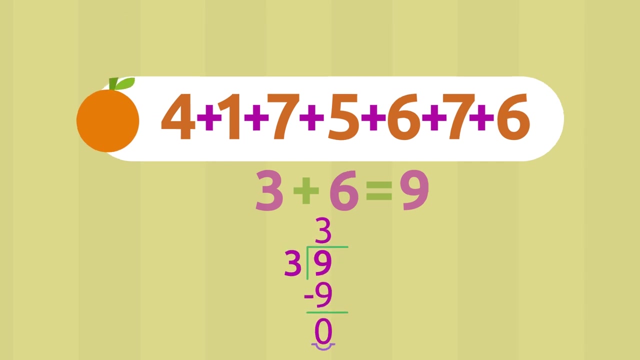 Let's test our theory by adding its digits. Nine is a very small number and we know that if we divide it by three, the remainder will be zero. The divisibility rule of three is super fun because we can add digits as many times as we want. 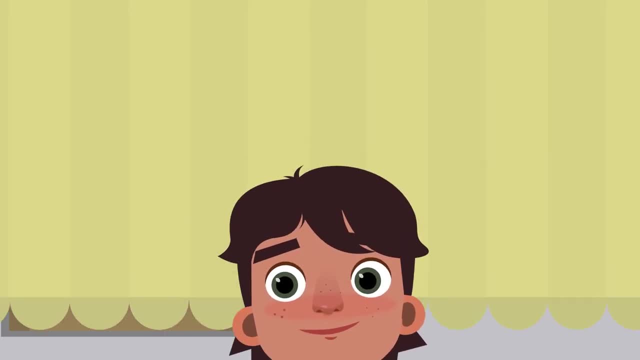 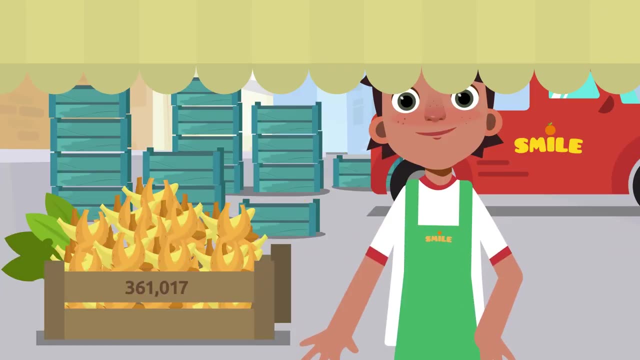 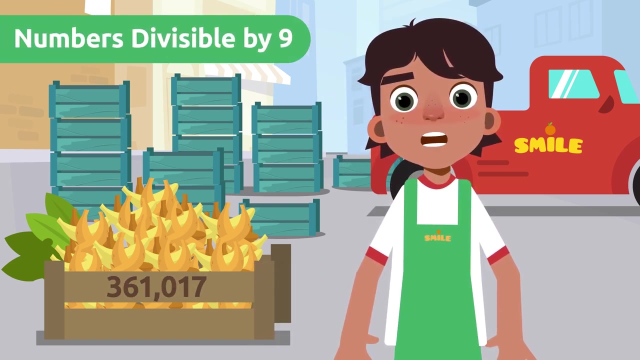 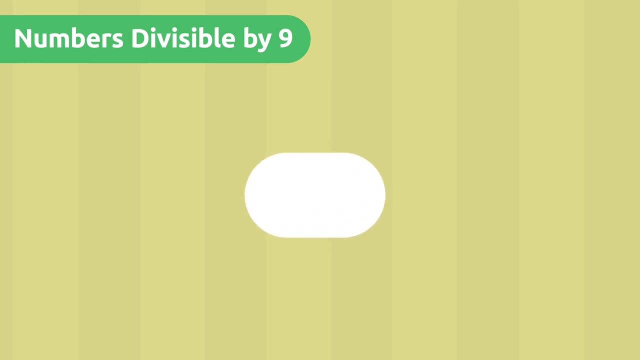 Isn't it very useful? We also send bananas. They are very healthy. There are three hundred and sixty-one thousand and seventeen bananas and we'll send nine per box. Let's see if we have any left over. The divisibility rule of nine is calculated in the same way as the number three. 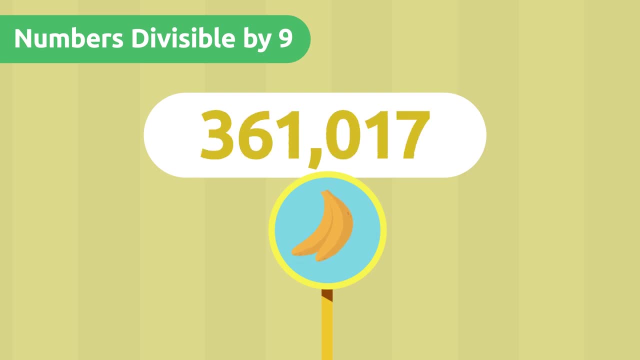 We have to add its digits, divide the result by nine and check that the remainder is zero. Take a look: Three plus six is nine, Nine plus one is ten, Ten plus one is eleven, And eleven plus seven is eighteen. Now we'll do the division.